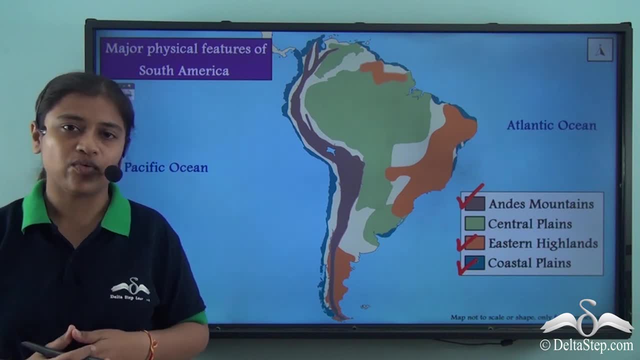 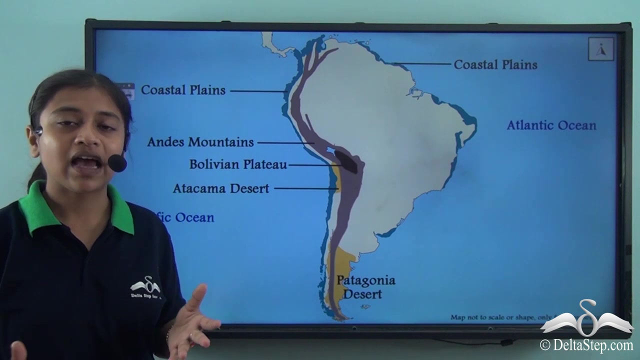 coastal plains of the continent are very narrow right, But they do have an influence on the climate and other aspects of the continent. So we can see here that the coastal plains are quite narrow and the west coast is almost devoid of any plains. This is mostly because the Andes mountains rises from rises very 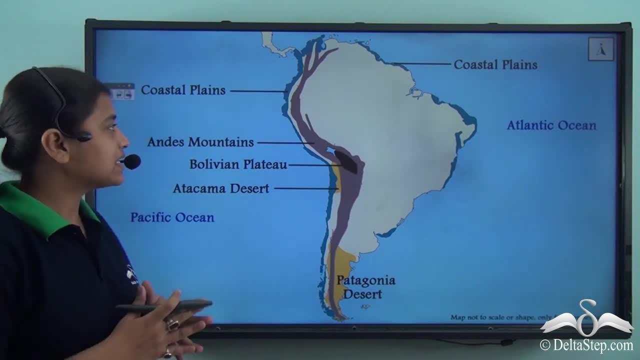 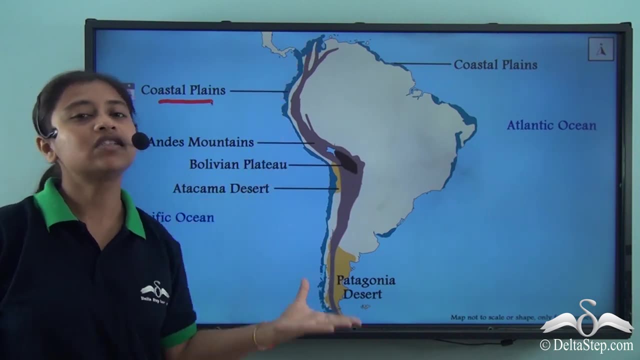 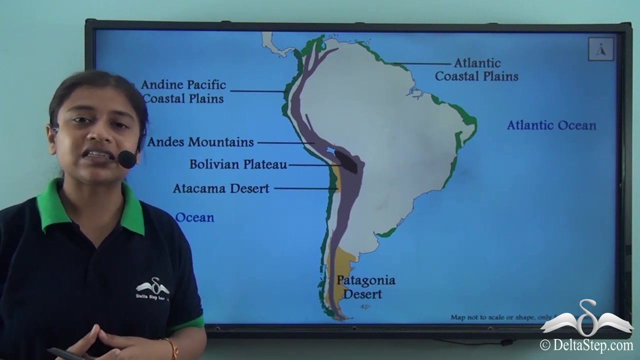 closely and steeply from the coast itself. So we can see that the coastal plains run on either side, on either coast of the continent, from north to south. Now the coastal plains can be broadly divided into two, That is, they can be known as the 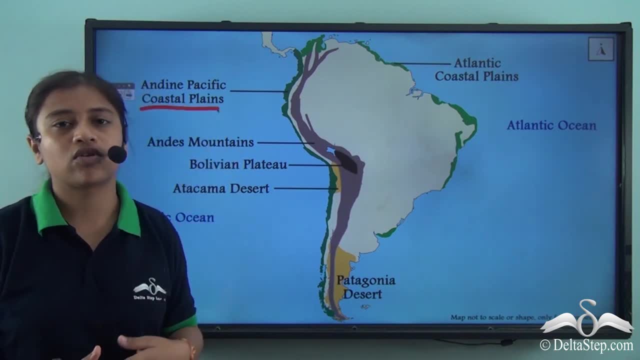 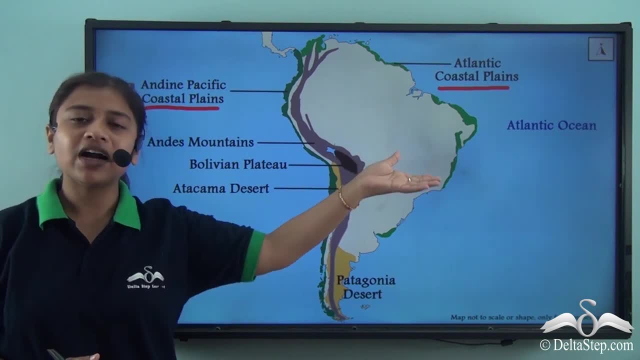 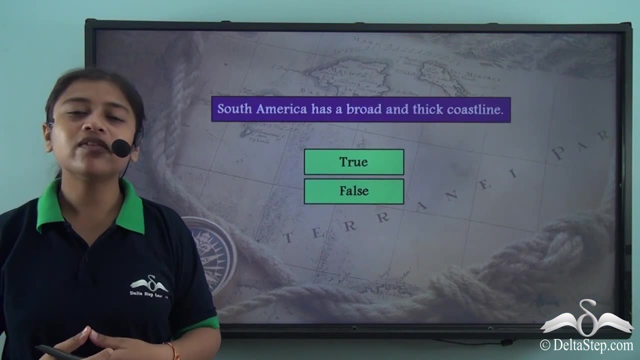 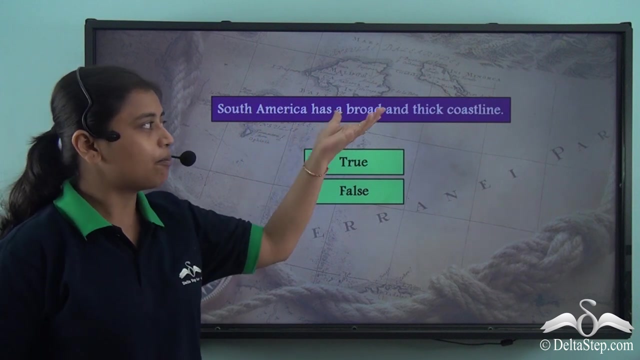 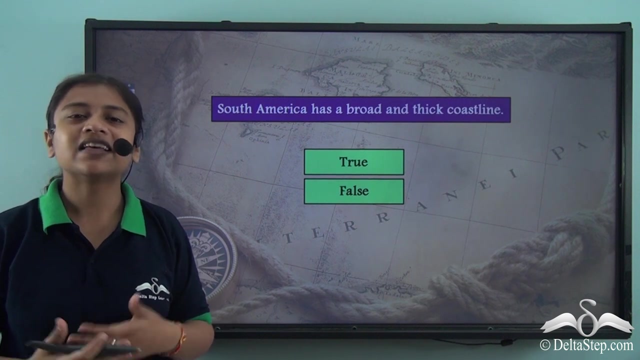 along the entire stretch of the western coast and partially in breaks on the eastern coast of the continent. So, before we proceed with the lesson, could you state whether the given statement is true or false? South America has. South america has a and thick coastline. Is it true or is it false? Yes, the correct answer is it is false, As 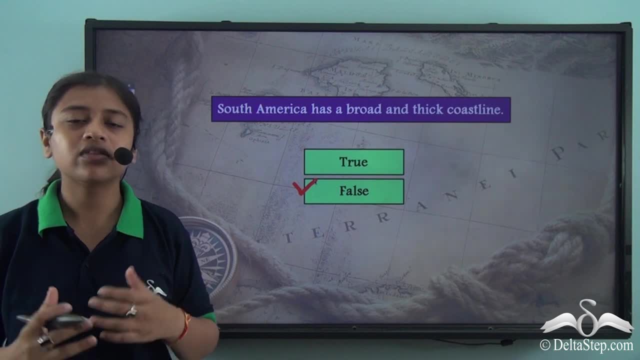 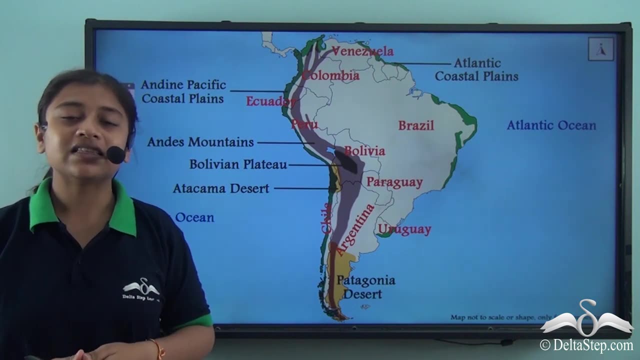 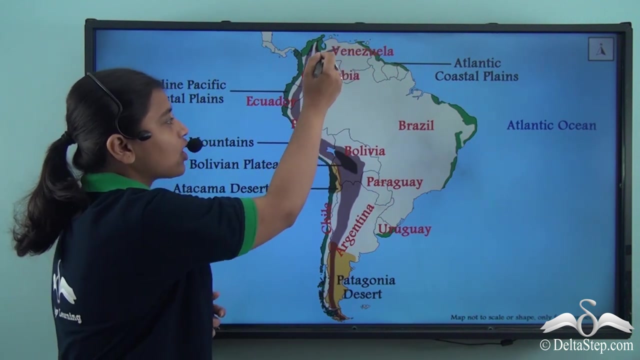 we have been learning that the coastline of the continent of South America is quite narrow. Now, moving on, we see that the coastline covers and passes through most of the countries of the continent, starting from Venezuela, Colombia, Ecuador, Peru, Chile. However, there are three. 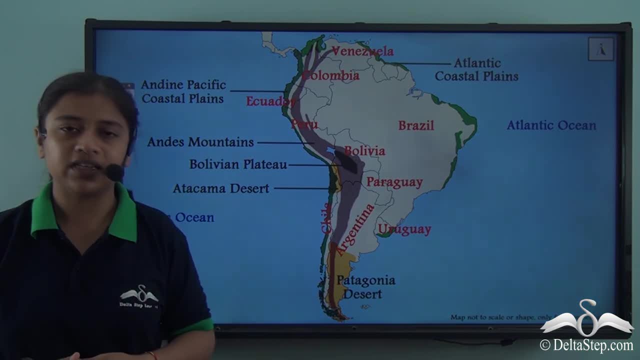 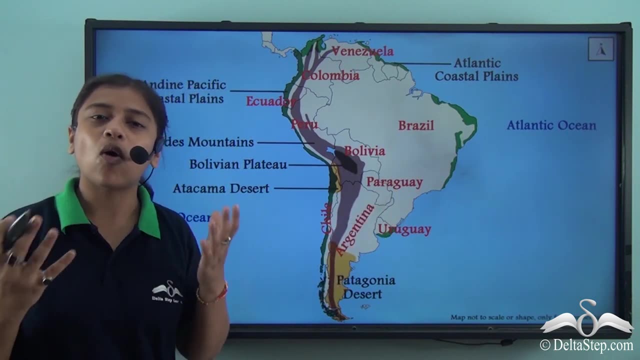 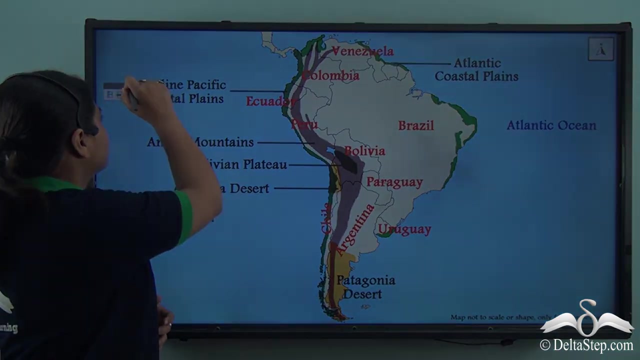 countries that are not quite influenced by the coastal plains, and these countries are Bolivia, Paraguay and Argentina. So we can see that almost all the countries, except these three, come under the influence of the narrow coastal plains. Now, these narrow coastal plains are fertile. 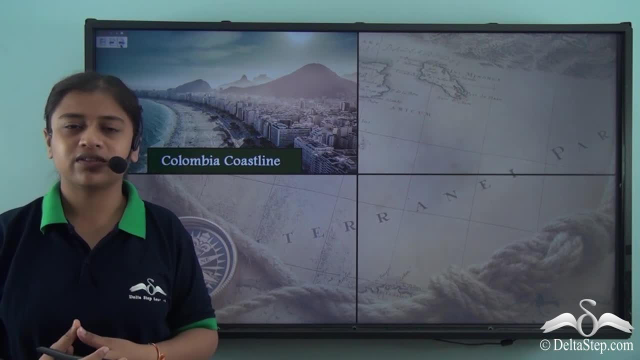 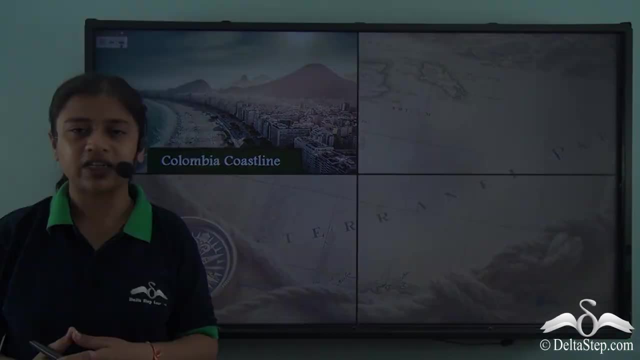 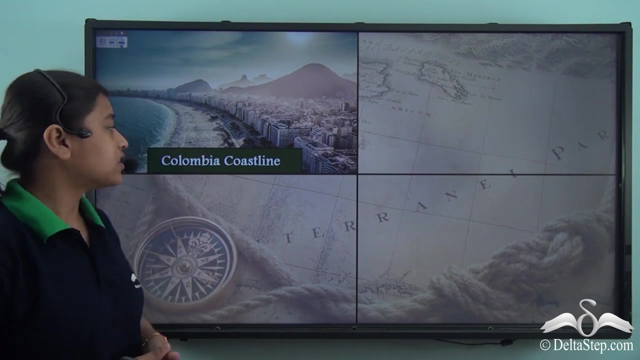 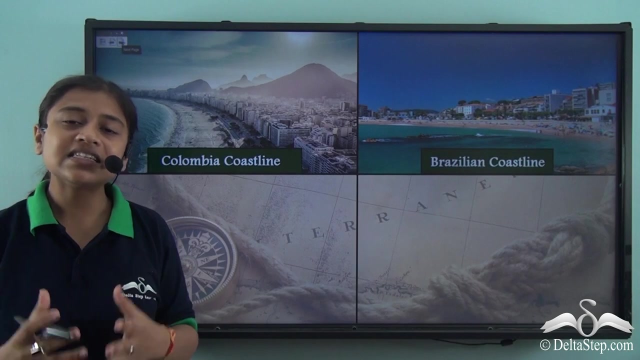 And they provide good grounds for agriculture and cultivation. Now, other than that, the coastal plains also play a very important role in the tourism industry of the country. These are some of the most famous and visited tourist attractions of the continent of South America, Be it the Colombia coast, the Brazilian coast. they are narrow and they are seasonally populated. 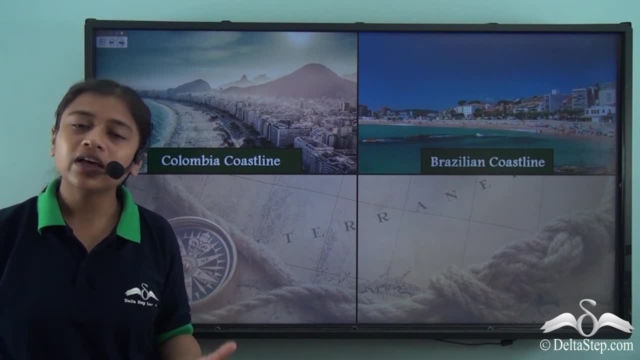 by tourists from across the world. We also have two other important places to visit in Colombia. The first is the coastline of the continent of South America. The second is the coastline of the continent of South America. The third place is the beach of the怎麼 beach. 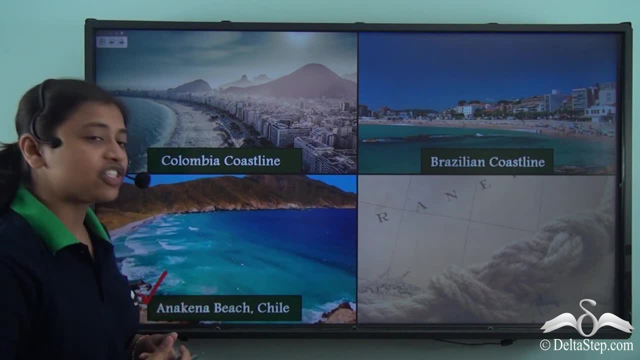 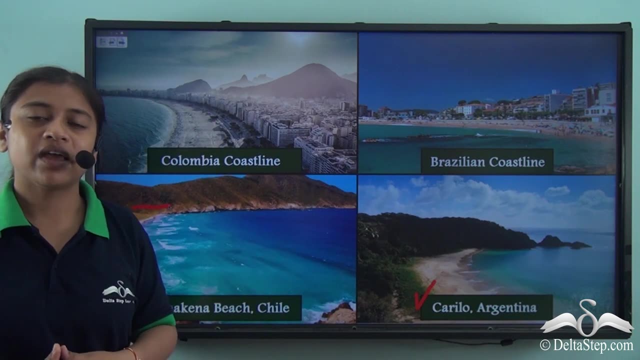 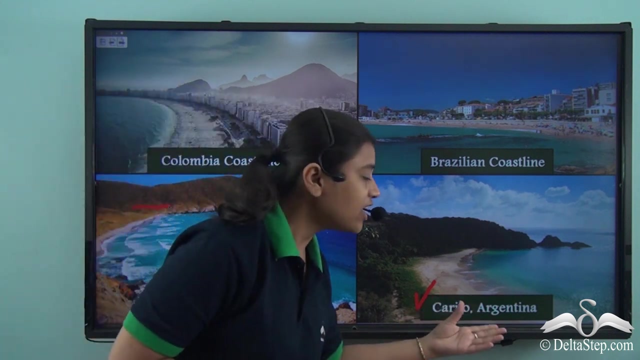 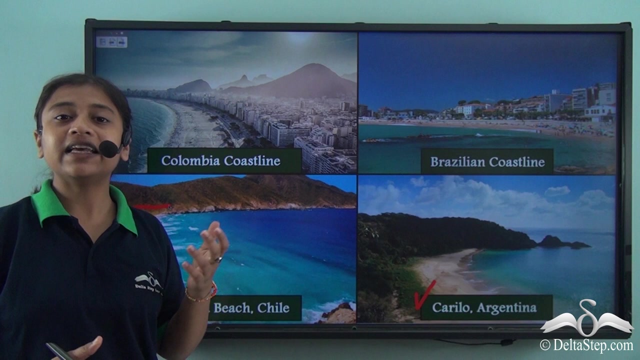 You can also visit the beach of the ery island. The fourth place is the beach of the Garibaldi. So the beach of Garibaldi is not only a beautiful beach, is also a great water park. So do you wish that you visit the beach of Garibaldi? Now, the beach of Garibaldi is also known for its warm turquoise water and white sand. The Carillo is a famous and one of the most visited beach resort town in Argentina, So we can see that these coastlines do not only provide fertile grounds for agriculture, but 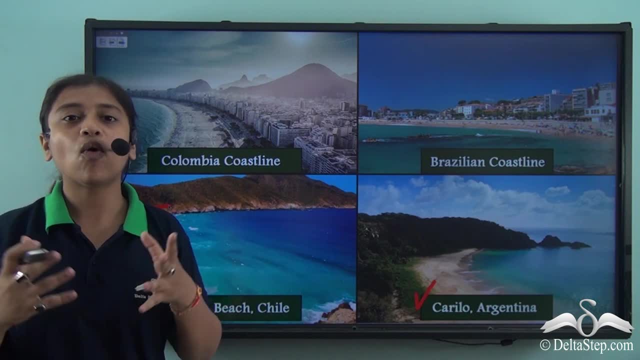 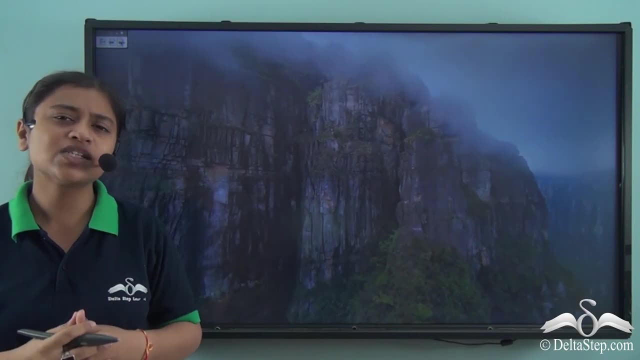 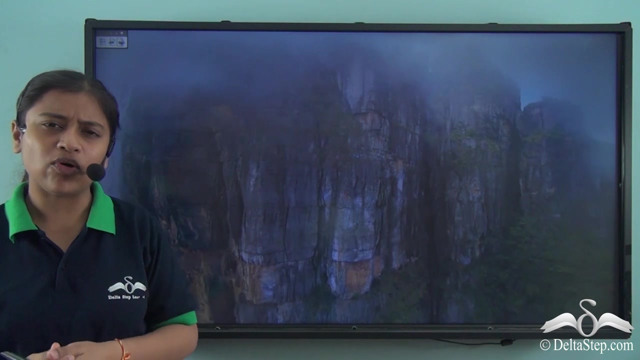 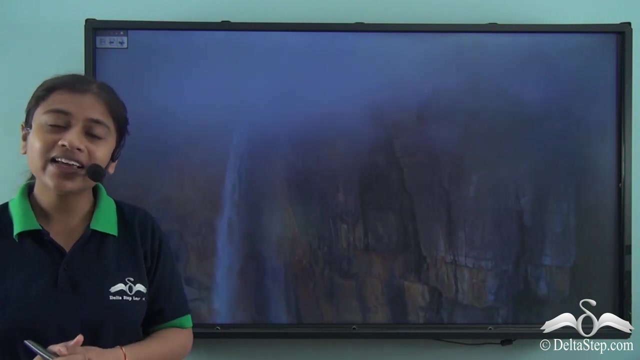 agriculture, but they also play a very important role in the overall economic boost of the country. Now, here we have the world's highest waterfall. Do you know what we are talking about? We are talking about the Angel Falls. The Angel Falls is estimated to be at a height of 979 meters. It is world's highest. 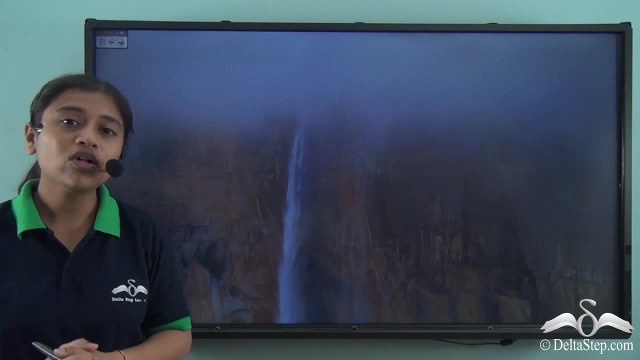 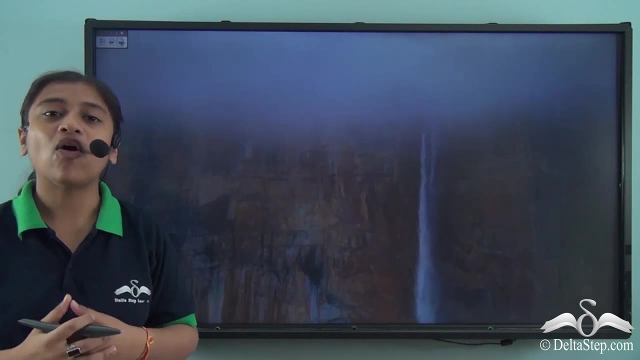 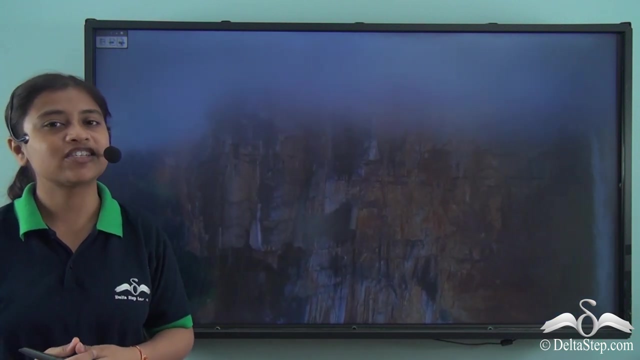 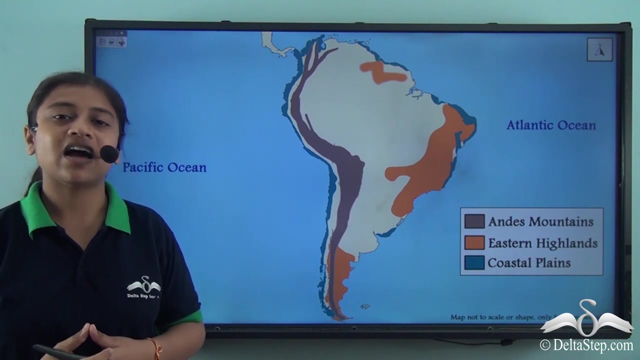 waterfall and is a spectacular view for all the tourists coming from across the globe. Now, where do we find this Angel waterfalls? It is just a part of the Guyana Highlands. Now, Guyana Highlands are another important physical feature of the continent of South America Now. so Guyana Highlands are just a part of. 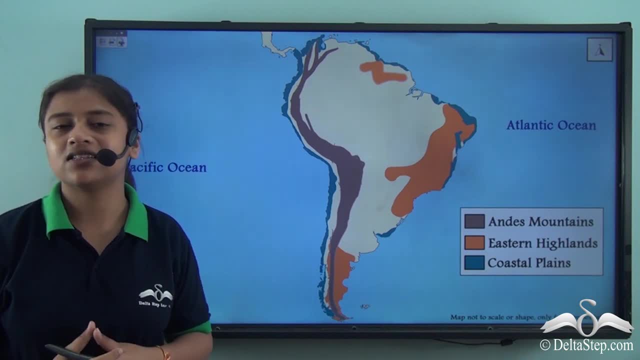 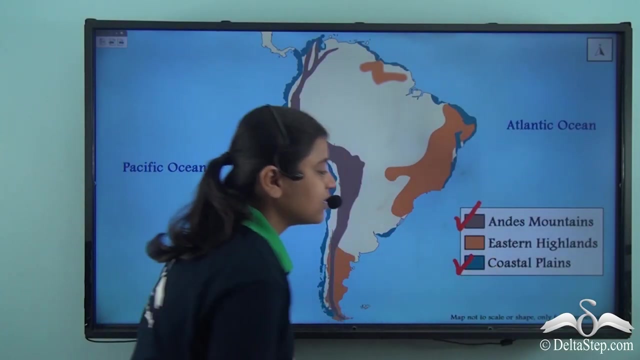 another physical feature of the continent, that is, the Eastern Highlands. Now we call them eastern highlands because they simply lie on the eastern part of the continent. In our previous lesson we learnt about the Andes mountains, and now we learnt about the coastal plains. 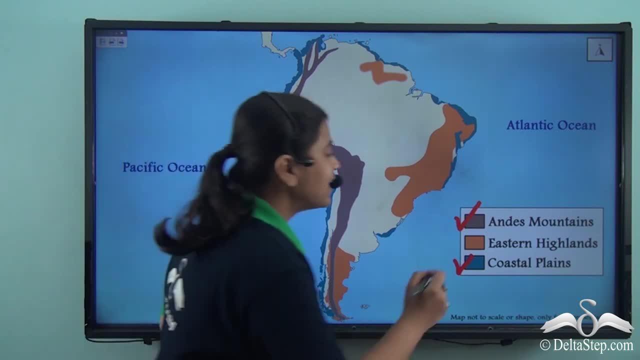 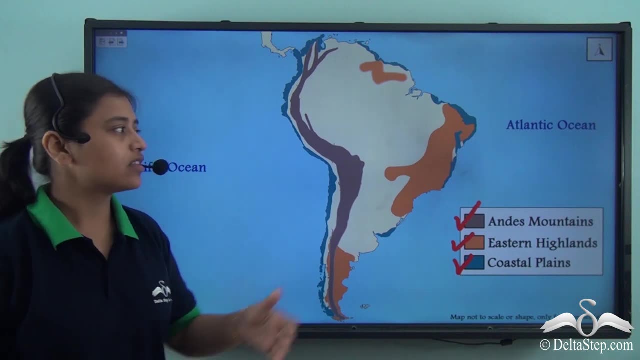 So let's proceed with the discussion by focusing on the eastern highlands. So the eastern highlands are just another important physical feature of the continent lying on the eastern part of the continent. As we can see, these highlands are not continuous. they are broken down into three. 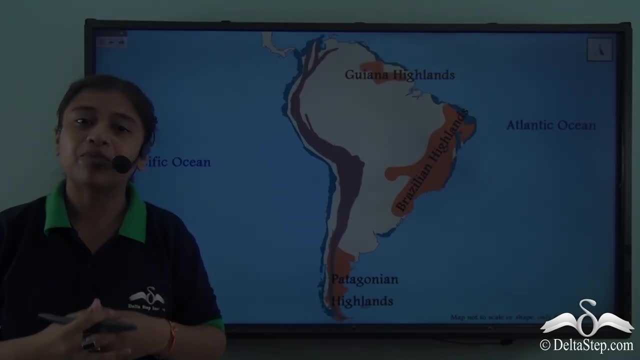 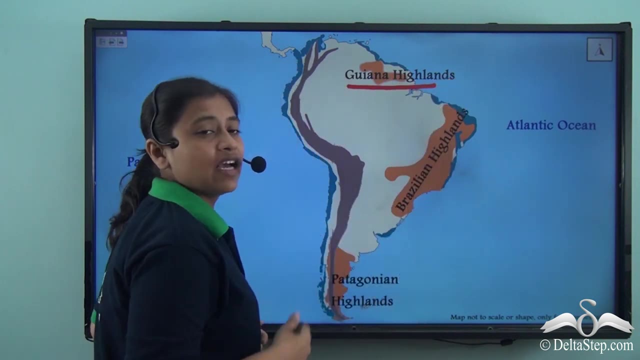 So the eastern highlands of the continent of South America can be broadly classified under three headings. They are known as the Guyana highlands, to the north of the continent, then they are known as the Brazilian highlands, being the largest highlands among the three. and finally, 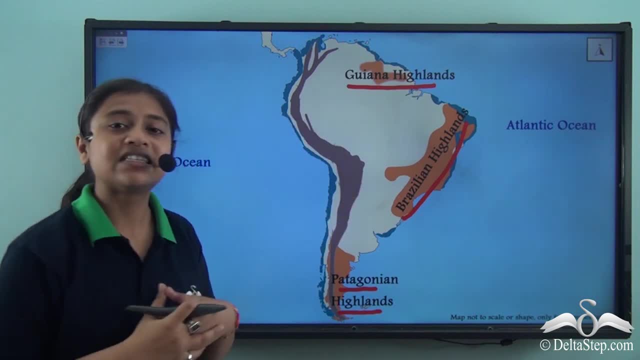 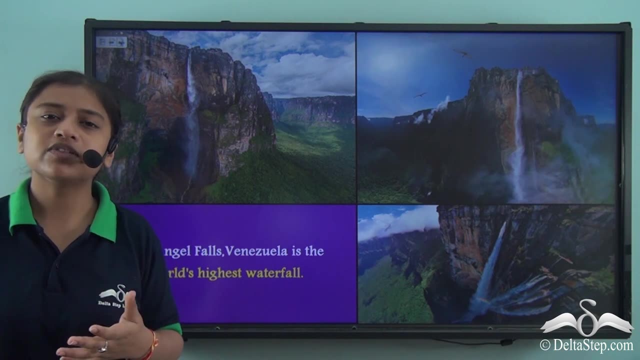 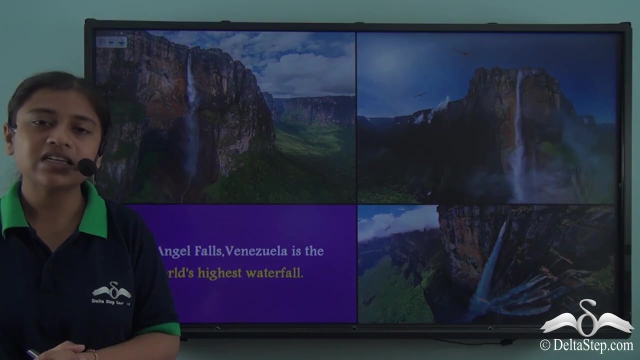 we have the Patagonian highlands, to the very south of the continent. Now these Highlands provide table top which are responsible for various important waterfalls. They not only are used for the production of hydroelectricity, but they also serve as famous tourist attraction. 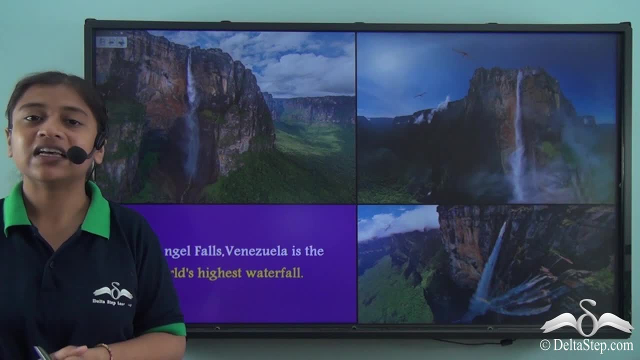 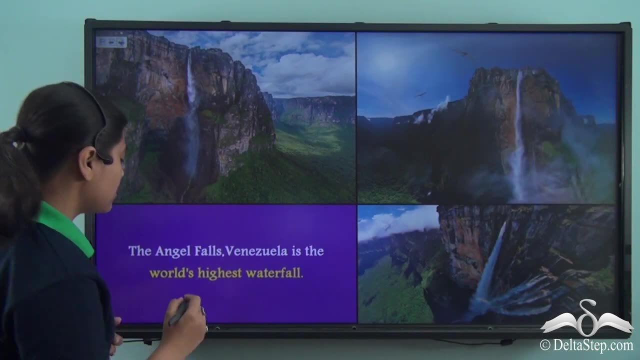 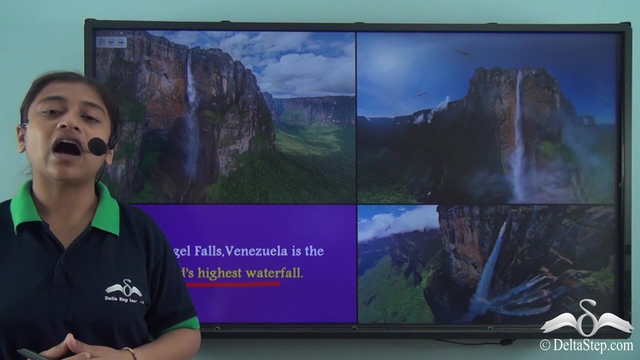 Among all these waterfalls, we learnt about the angel falls. The angel falls provides a spectacular view of the place and it is in Venezuela and, as we learnt, it is the world's highest waterfall, a height of 979 meters. Now the Angel Falls are a part of the Orinoco river system. Now 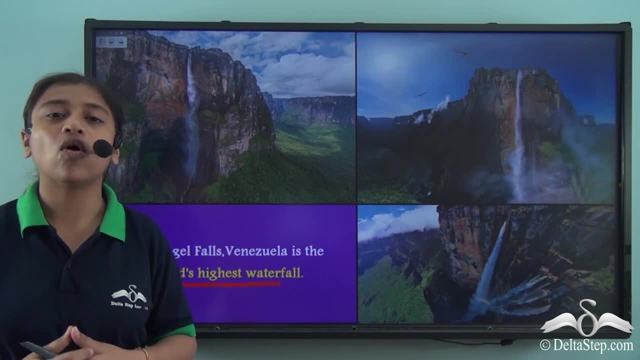 Orinoco river system is one of the most important river systems of the continent of South America, and this river system is what we will be learning as a part of the fourth physical division of the continent, and that is the central plains. So in this lesson we were able to learn about